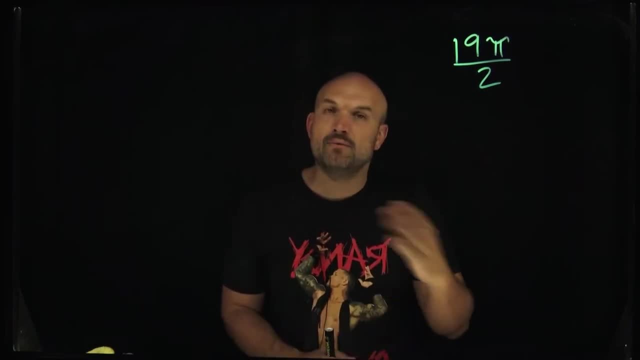 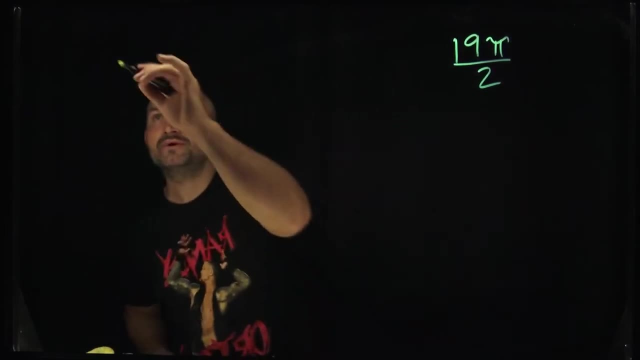 of like a number, as well as how do we graph that in standard form and what point does that correlate on? So there's a lot that we need to know. I think the first thing we need to do is break up the 19 pi or 19 over 2.. Forget about the. 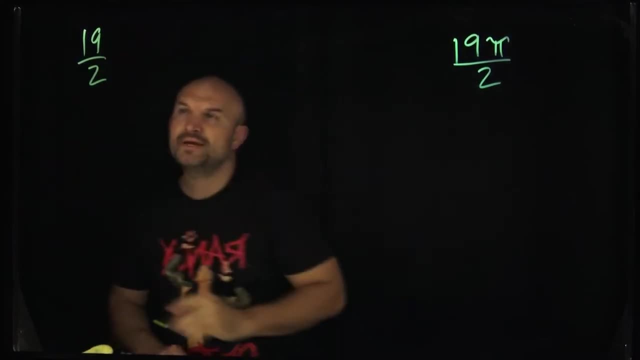 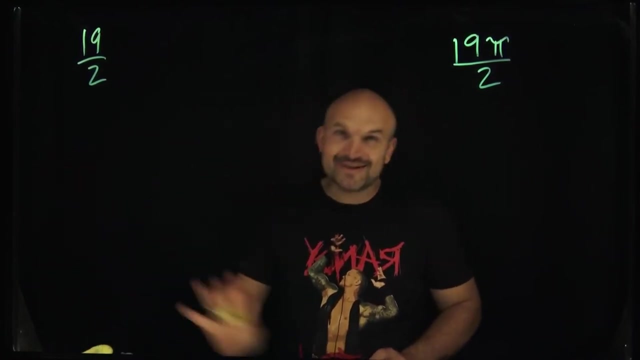 pi for a second. Let's just forget about radians, Let's just take a 19 over 2.. Alright, now that is an improper fraction, and maybe you remember in like the good old days, like when we did fractions like: oh yes, just even fraction, no letters, no. 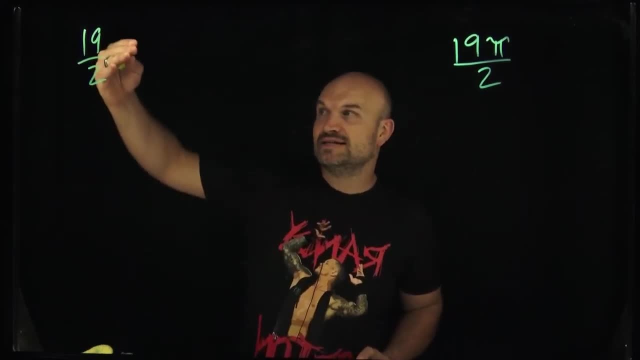 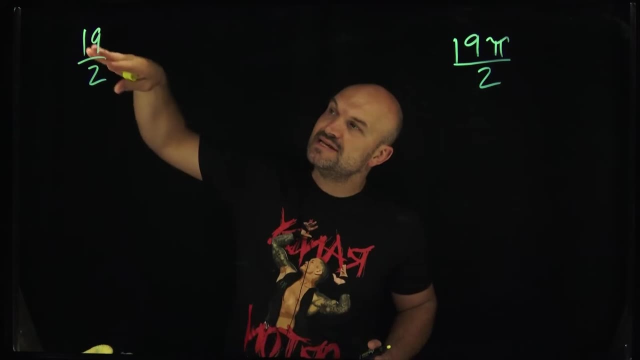 radians, decimals, just fractions. One thing we talked about was we like to convert improper fractions into what we call the mixed numbers. right, and the way to do that was we took our denominator and said: alright, how many times does that evenly divide into our numerator? and you could say: in this case that is. 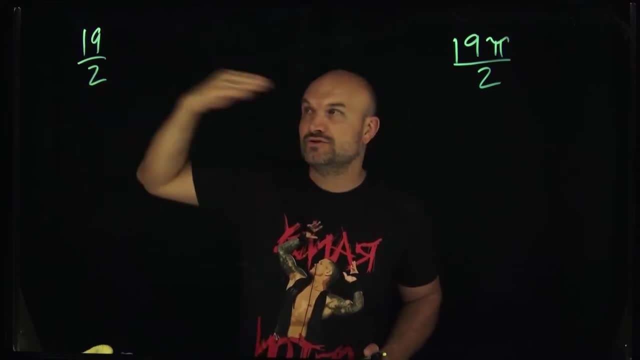 going to divide into our denominator, So we're going to divide that into our interior there nine times right. and then we took the remainder, which would be not 2 times 9, is going to be 18, so it has a remainder of 1, and then we put: 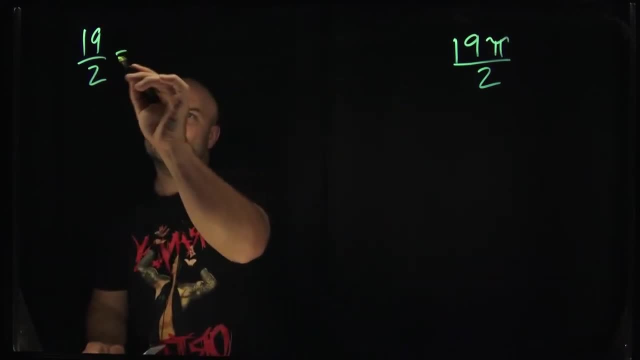 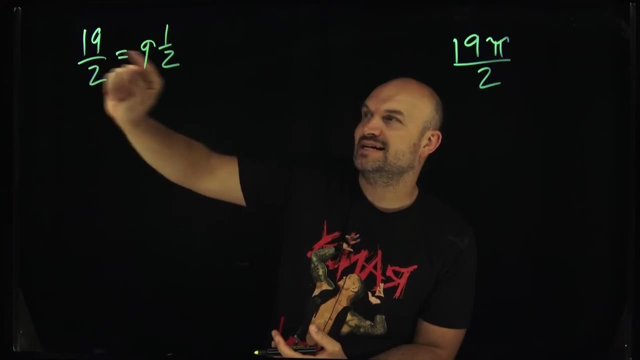 that in the numerator and then we keep the denominators 2.. So therefore, I could rewrite this as a 9 and 1, half right, and let's go and see like that makes sense, hopefully, and you can see like 2 goes into 19 nine times with the. 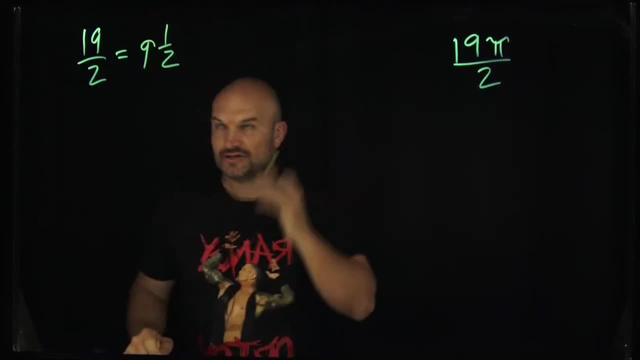 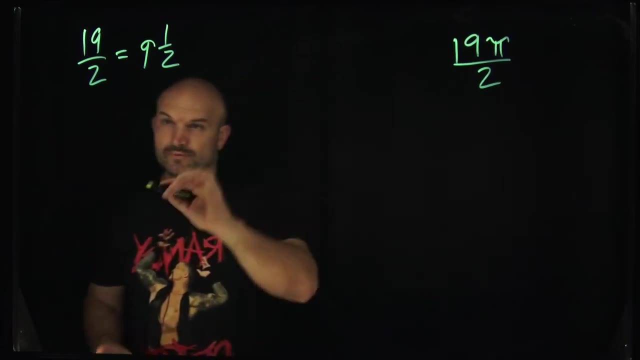 remainder of 1.. Okay, so this is our mixed number, that is our improper fraction. So how does this represent? because we don't really talk about radians in terms of mixed numbers. right, that's kind of weird. So one thing you need to understand about when we're dealing with: 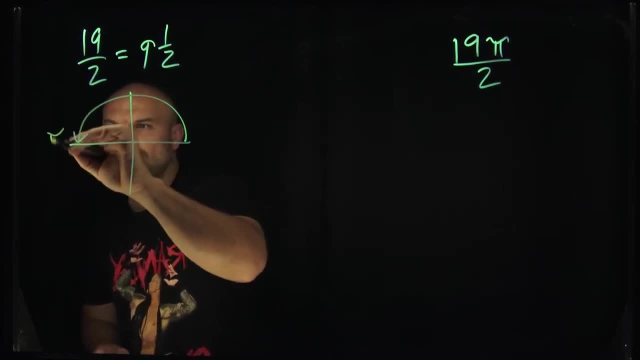 radians is like: remember, halfway around the circle represents pi. all the way around the circle represents 2 pi. okay, Now, we usually don't write a 1 in front of this, but that's something I want you to understand. like halfway around is like 1, all the way around, be 2. right Now, you can keep on going this extra. 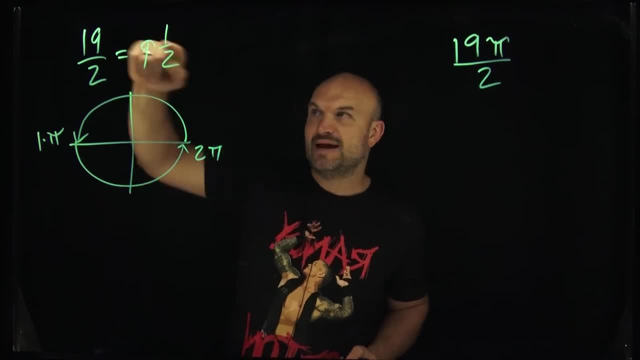 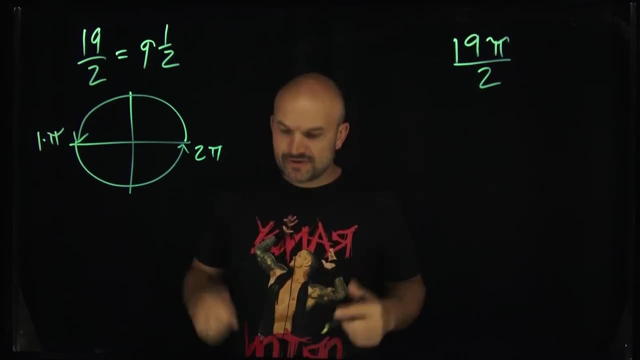 revolutions in this case. So what I want you to kind of see here is: we have this 1 half. I want to be able to rewrite this number in something that's probably maybe a little bit more familiar to what I have, and to do that, what we need to. 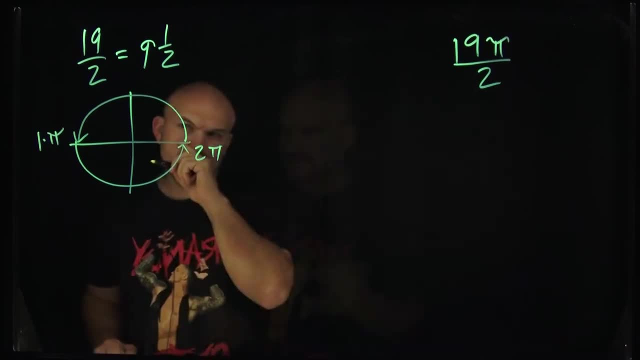 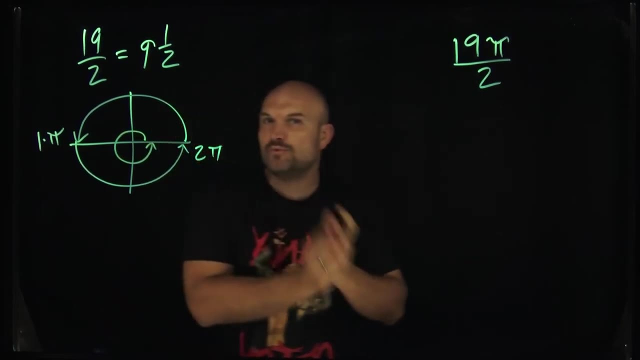 understand is like what happens when we have these extra revolutions, right? The thing that's important about when we're dealing with angles that are larger than pi. you need to understand, like, if I go around the circle once, like I'm back to where I started. right, that's what we 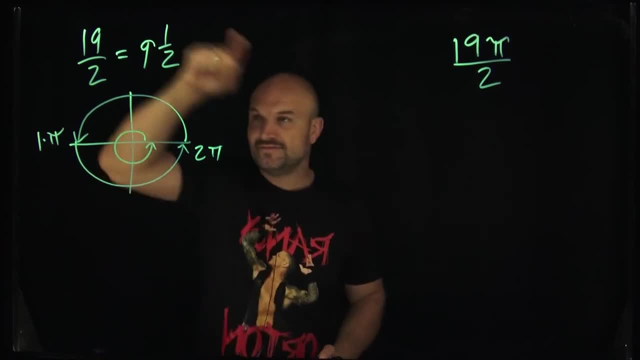 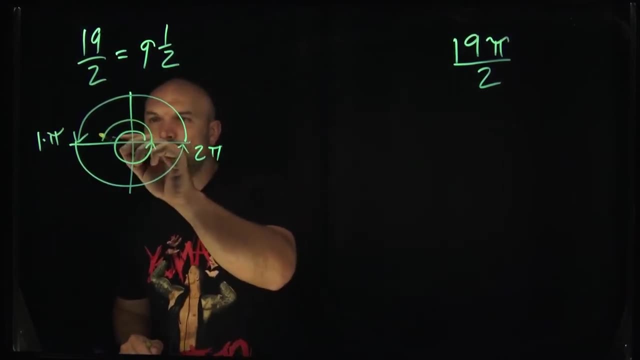 call like a revolution of pi. So as long as you're going around an even number, okay, you're just back to where you started. However, if you go around an odd number, right, if I just say, like you know, an extra 1 rev, like or not 1, right you? 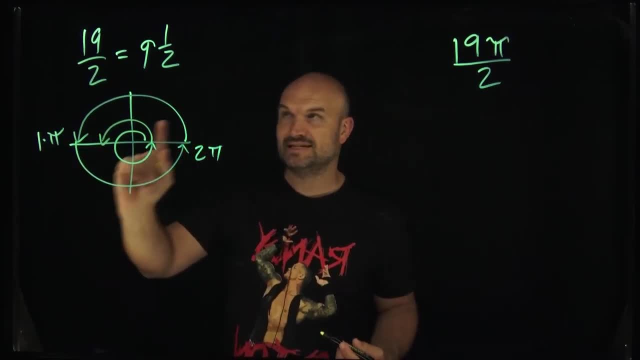 can see I'm over here. I'm on the negative version of this x-axis. that's gonna be something different. So what I want you to do is say like: alright, well, I have an extra 1 here and I want to rewrite this as a 2 and I'm gonna count. 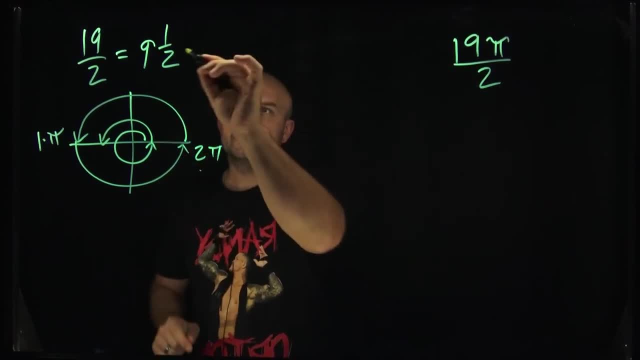 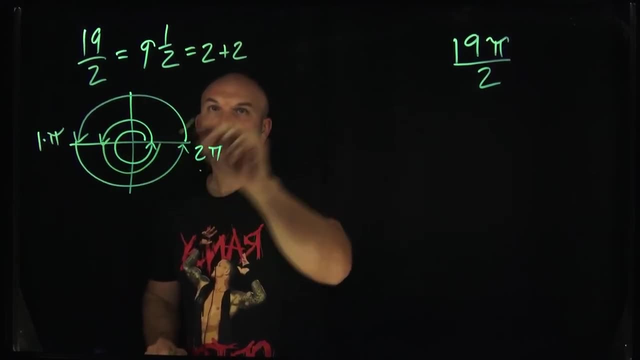 my revolution with this, right? So again, forget about the pi for a second. just kind of think of, like, whatever the number is in front, that'd be a revolution. So therefore I could rewrite this as a 2: that'd be 1 revolution plus 2, that'd be another revolution, right? So let's go around: 4 plus 2, it'd be another. 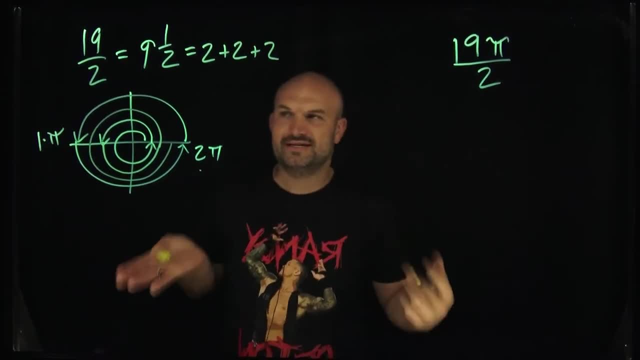 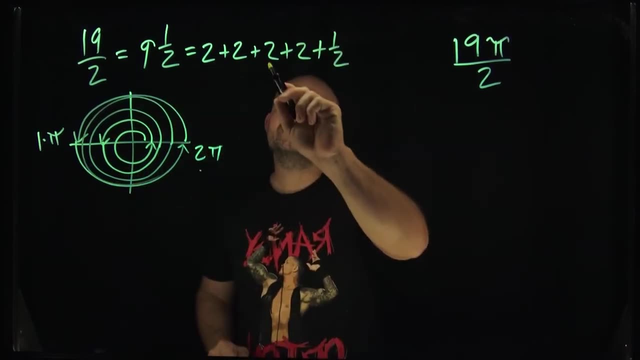 revolution, right. So now we're on 3 revolutions, But again, like it doesn't matter, even if I counted it wrong, like 3 or 2, like it doesn't matter, we're back to where we started. right, 2, 4, 6, I can go around another right. So 6, 2, 4, 6, 8, right. 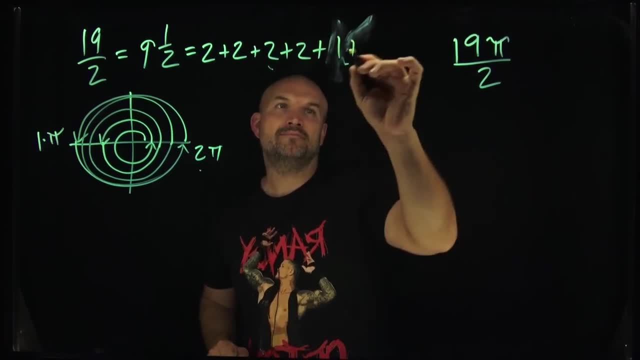 and then I can make a new one. So here we have, here's 4 plus 2 plus 3 plus 6, that's our revolution. we get. I gotta add a one plus a one half, which is kind of weird. all right, 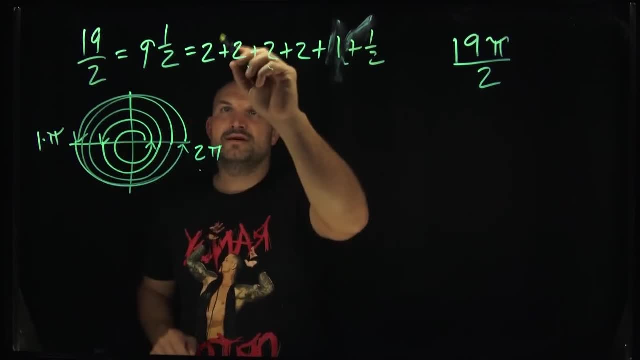 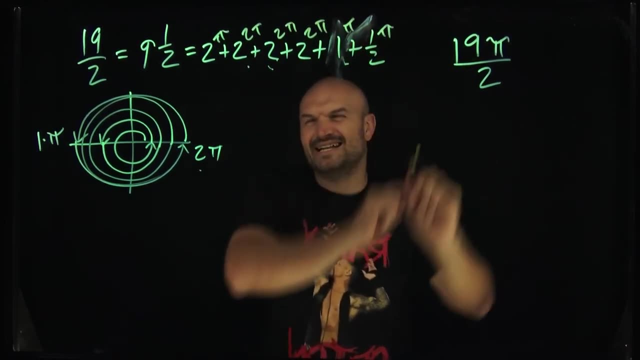 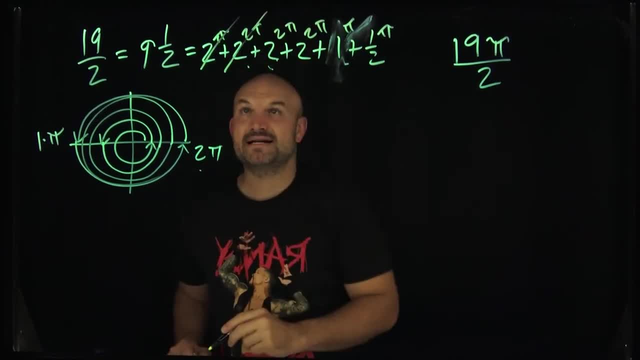 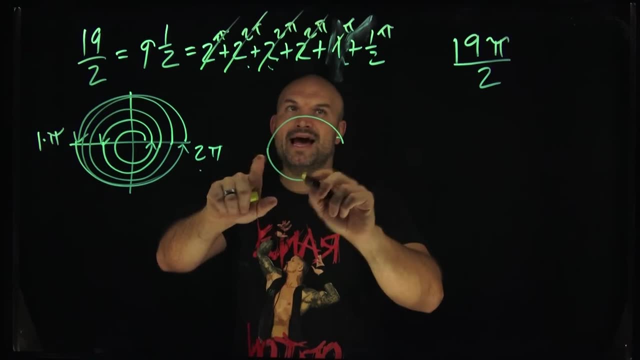 with these revolutions. Well, that's just taking us back to the beginning. That's taking us back to the beginning, back to the beginning, back to the beginning, back. And then here you could say: oh well, it's like a one and then a one half. 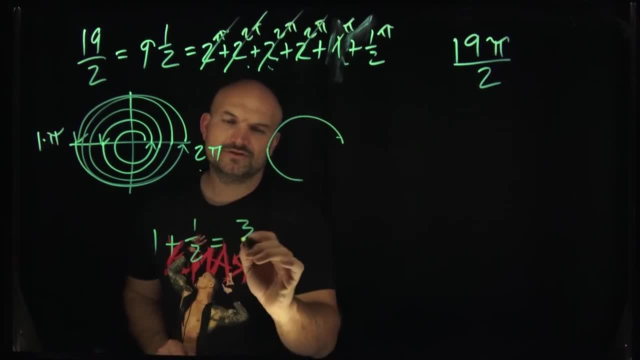 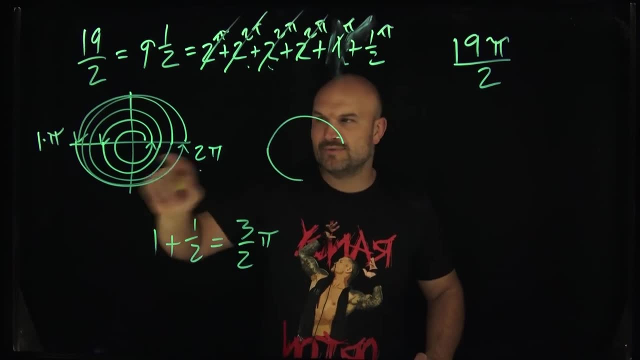 And again, like that should hopefully make sense: One plus one half is equal to three halves And hopefully you recognize that three pi over two right is represented by this coordinate point which hopefully would make sense. right, We did a revolution all the way around- which is two pi. 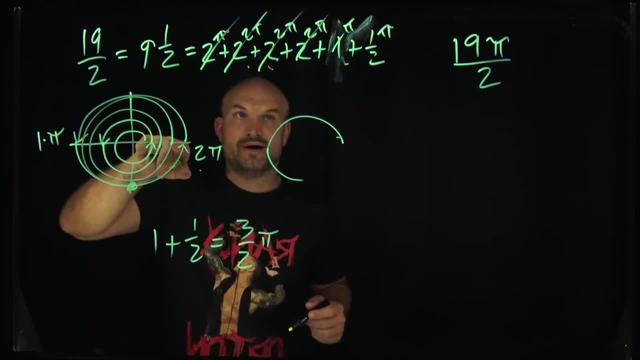 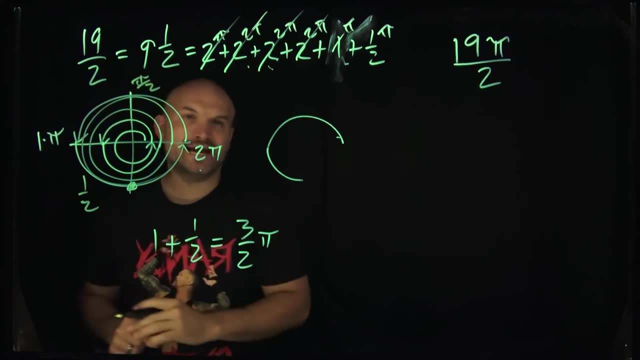 another revolution: two pi, another revolution, two pi, another revolution, two pi. Then we went over one pi and then in half right And you could see like, yeah, that's a half of a pi. So hopefully you can see how that makes sense. 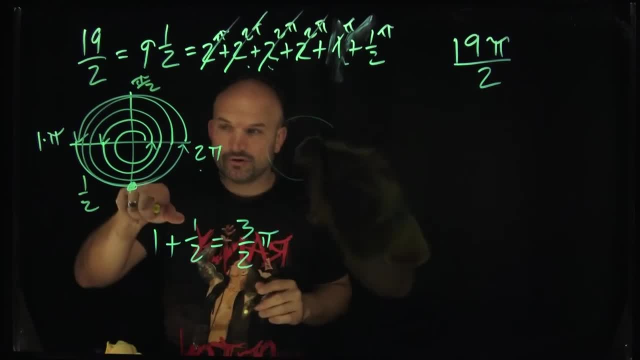 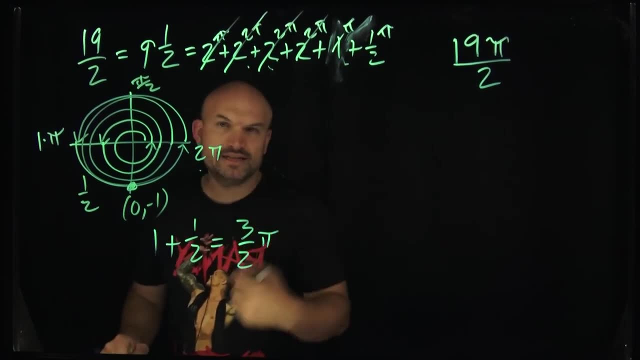 Now we just need to understand well, what exactly is. what is that coordinate point? This coordinate point is going to be a zero comma, negative one. So how do we now evaluate our six trigonometric functions from there? Well, remember when we're dealing with sine cosine. 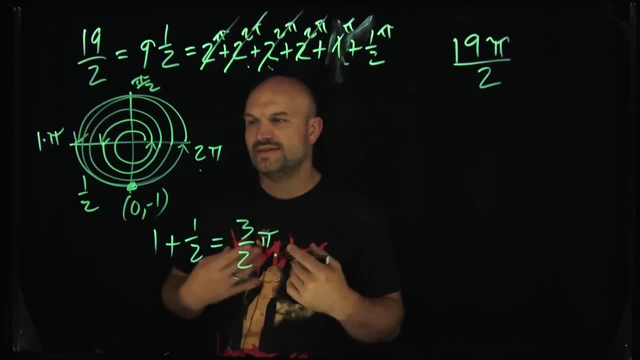 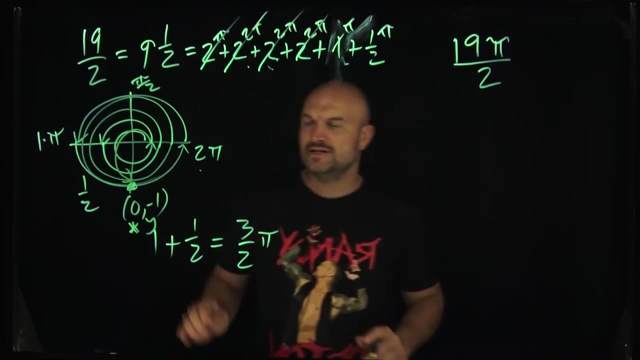 and tangent. we want to evaluate them on the unit circle. We're looking for the X and the Y coordinate of that point that lies on the unit circle for our angle, right, because our angle is going to end here. So you can see X is going to be zero. 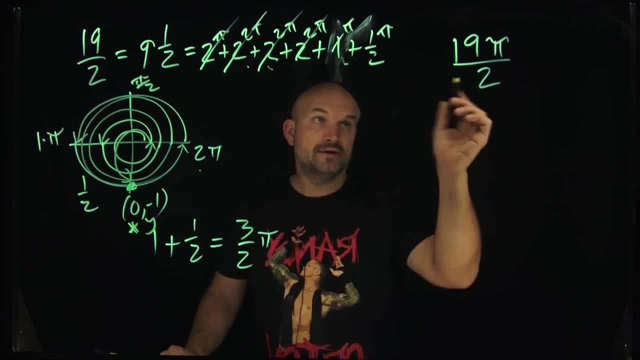 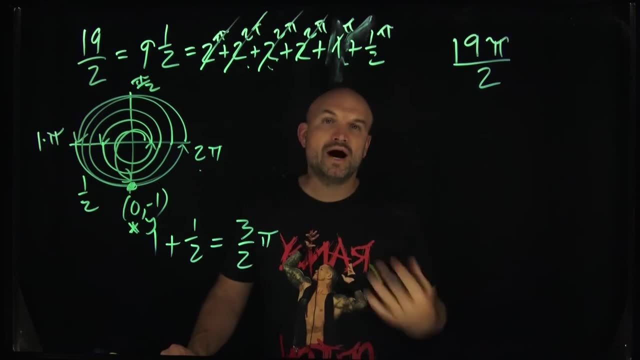 and Y is going to be negative one half. So the sine of our angle, 19 pi over two, is going to represent the Y coordinate, The cosine of 19 pi over two is going to represent it's X coordinate And the tangent is going to represent the Y over the X. 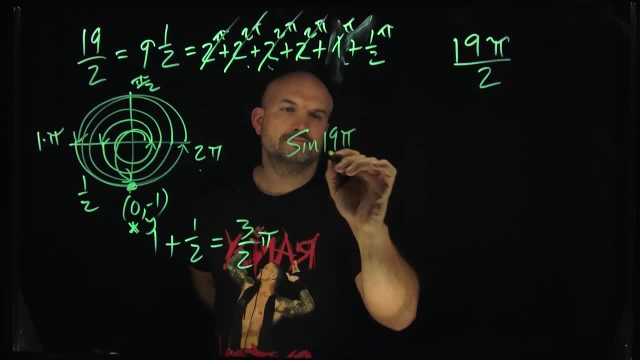 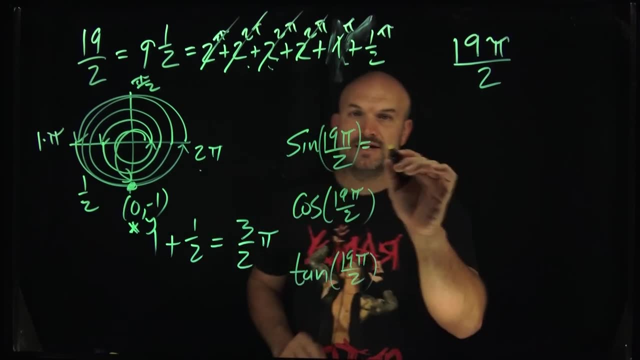 So let's go ahead and write all of those out, Okay? so remember, sine represents Y, So in this case that's negative. one Cosine of 19, pi over two represents the X, which in this case is going to be a zero. 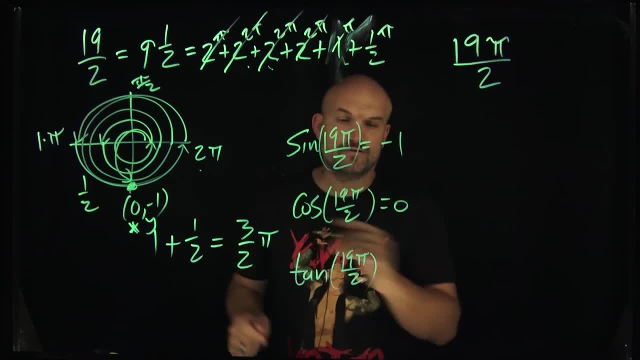 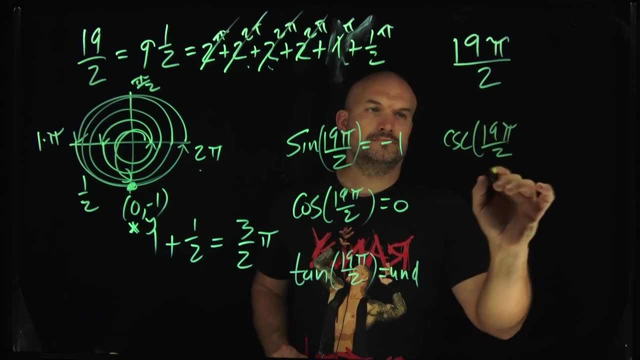 And the tangent represents the Y over the X. Notice that's going to be negative, one over zero. So therefore that's going to be an undefined. Now let's go ahead and do our reciprocal functions, Okay. so remember that's just going to be one over Y. 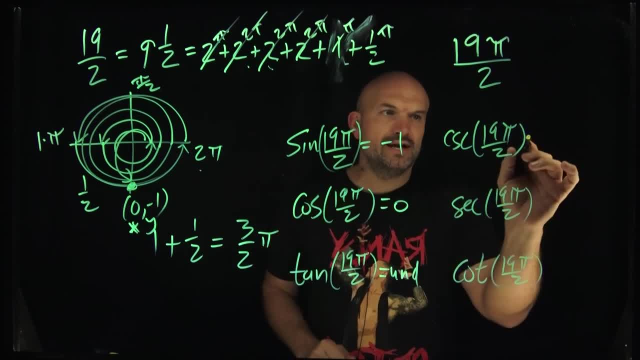 for the cosecant. So we have Y is negative one. So one over Y is going to be a one over negative one, which is just a negative one. If we go to secant, that's going to be one over X, right? 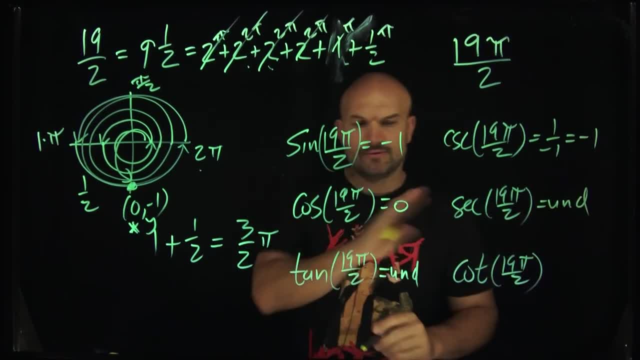 Well, X is zero, So one over zero is going to be a undefined. And then we'll go ahead and take a look at cotangent. That is going to be. now. a lot of times students are like: well, how do you do one over undefined? 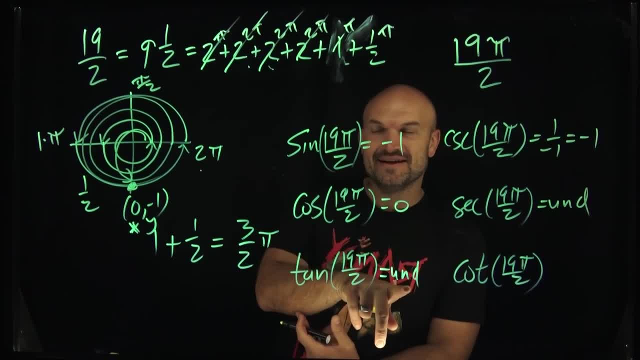 Like that has to be undefined as well. Yes, again, if you are thinking of this answer, but in this case let's go back and look at this. Let's go back to it: If tangent is Y over X, then cotangent is going to be X over Y. 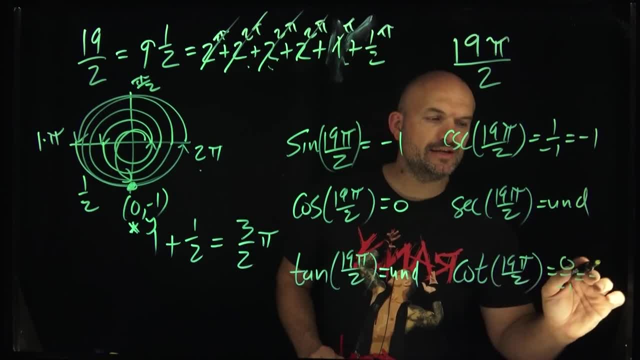 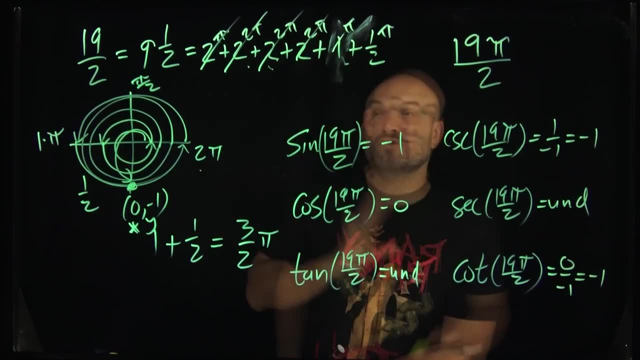 So in this case, you have a zero over a negative one, which is just going to equal a negative one. Now, this problem was difficult because we had a really, really big angle, But in the next video I'll go through the exact same process. for an angle that's so big we can't even graph it. 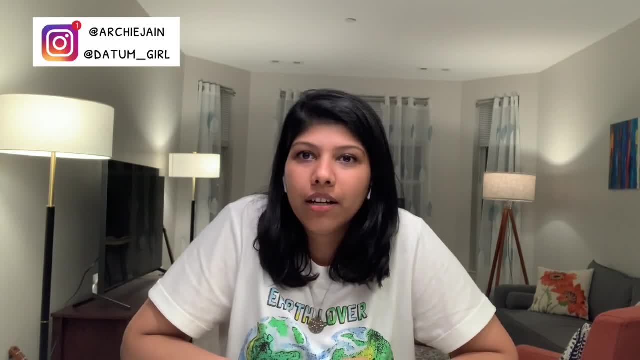 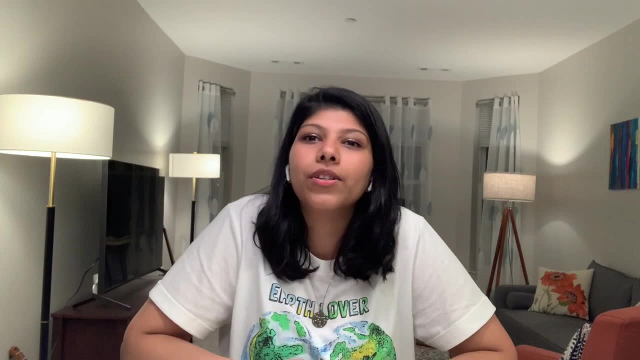 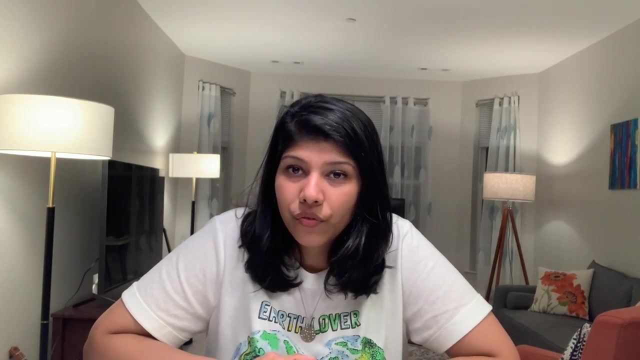 Hey guys, my name is Archie and I'll be posting some videos related to data science, data analytics, engineering and answering all your questions- anything that you have about data on fellow brownies channel alongside my own. So in this video I'll be addressing three main topics. First would be about my profile and my